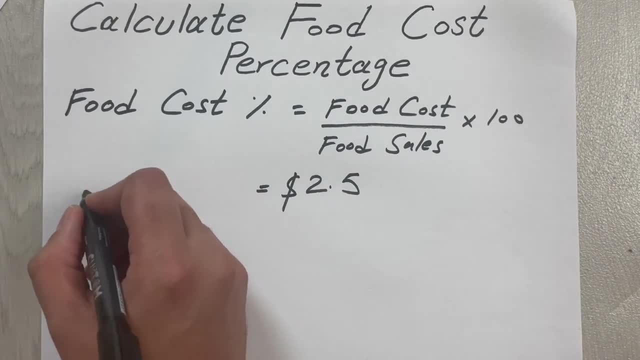 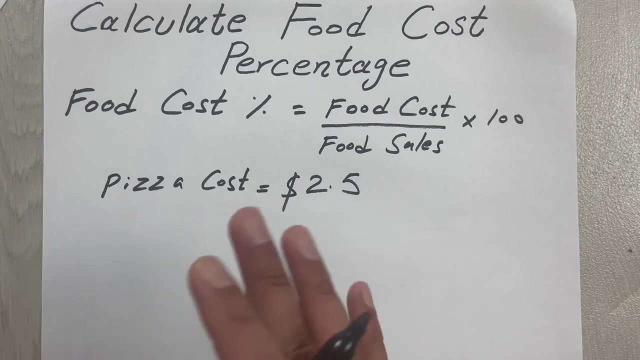 dollars or rupees, okay, so the pizza food cost, so the pizza cost is 2.5 dollars. okay, and let's say it include all the entire cost of producing the pizza, including labor, ingredients, everything in it, including this 2.5 dollars. okay, and let's assume we gonna sell that pizza. 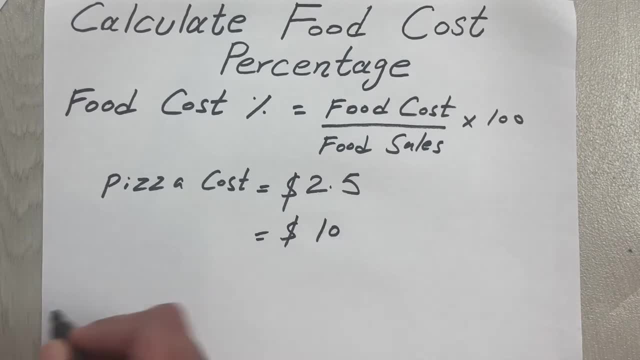 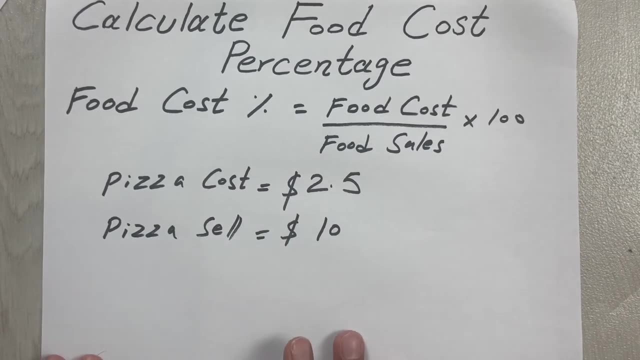 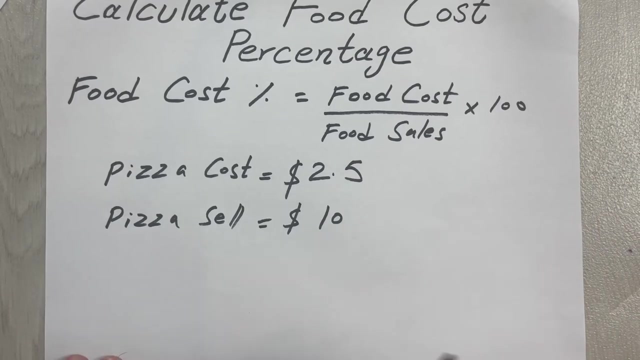 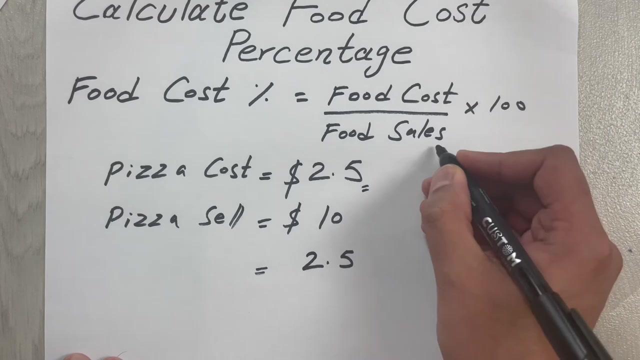 for, let's say, ten dollars. okay, so the pizza sell at ten dollars, okay. so now it is very simple. we can put the values into this formula and we will get our food cost percentage. so the cost food cost is 2.5 and the food sale is this: 10. so 2.5 divided with 10, multiplied with 100. 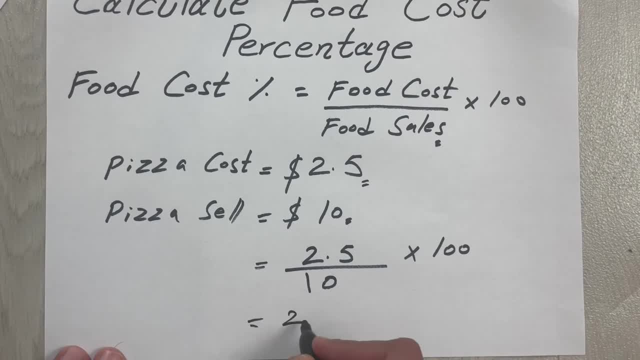 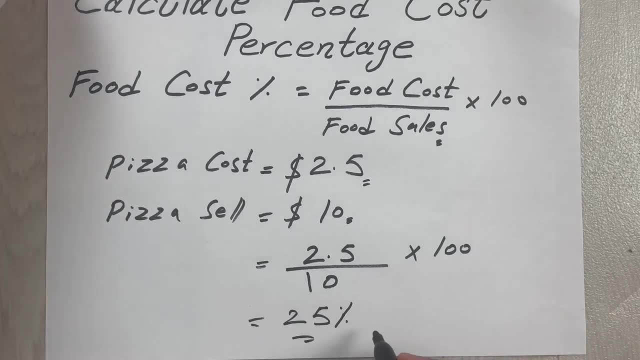 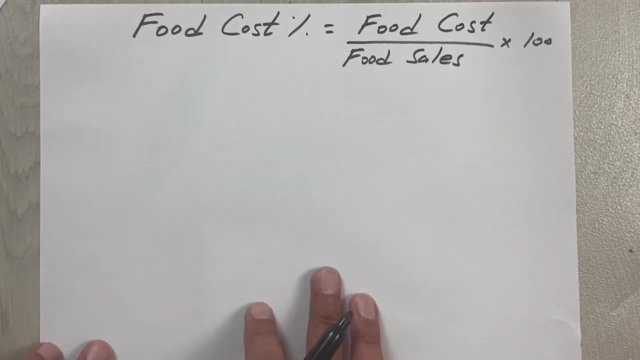 so when we do this calculation, our answer will come is to 25 percent. so, guys, this is our food cost percentage. so now it means that this 25 percent of the selling price will be allocated to the food cost. let's move to one more example. so, guys, i move to one more example. i already put the formula for the food cost percentage over here. 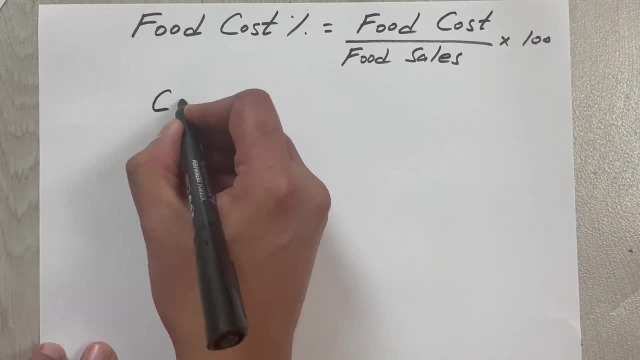 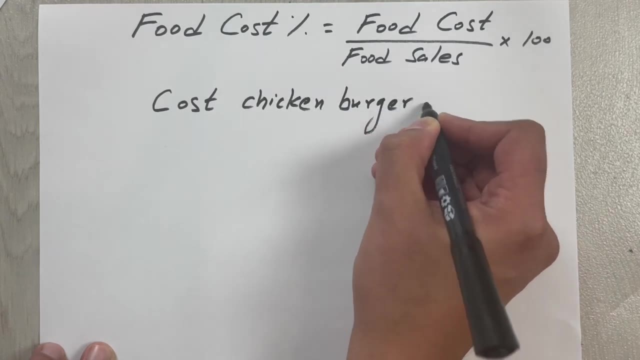 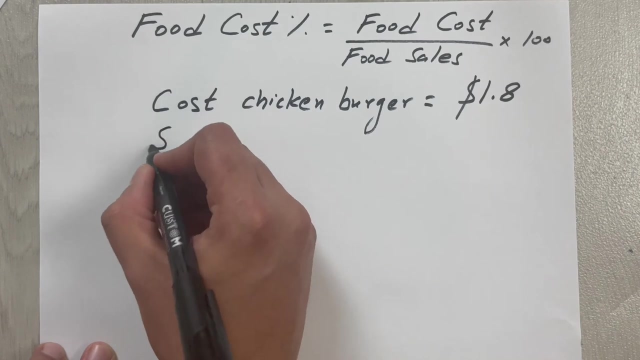 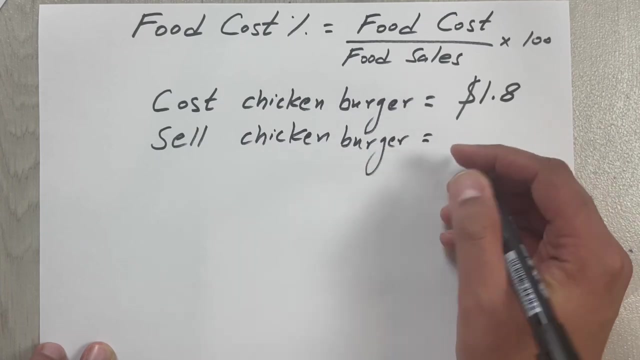 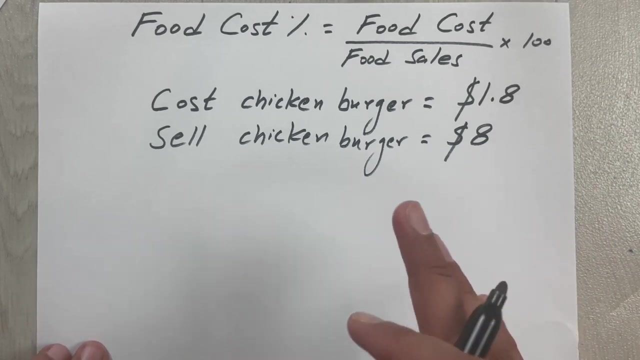 so let's say we have a chicken burger and the cost of that chicken burger is equal to 1.8 dollars or rupees or whatever currency you want, and you sell that chicken burger on, let's say, eight dollars. okay, so the cost is 1.8 dollars and with the selling price is eight dollars. 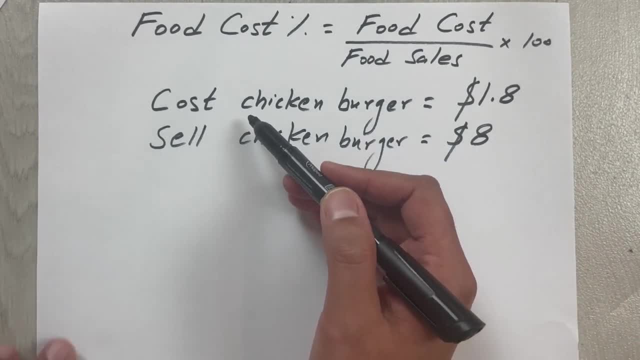 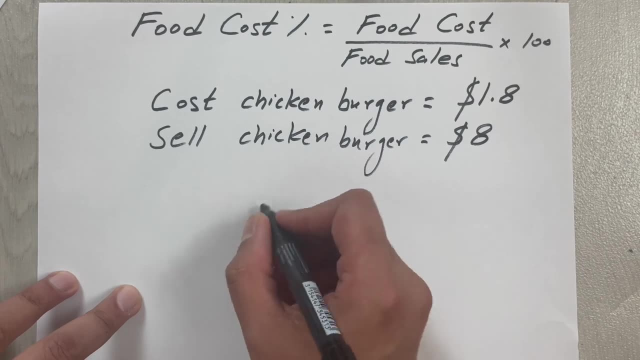 so this cost, as i already mentioned, it includes everything. it includes labor, the ingredients, the bills, everything. okay, so now this cost of chicken burger is 1.8. so now we will put the values in this formula, which is very simple: 1.8, which is the food cost. 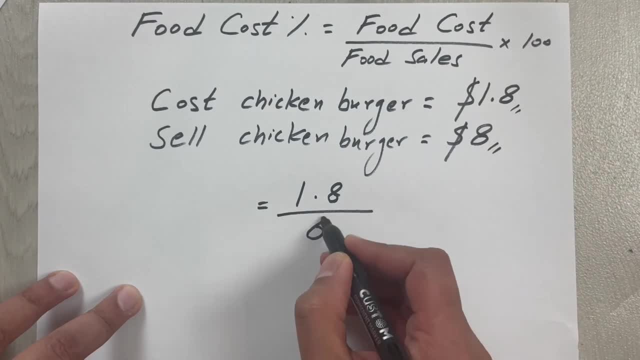 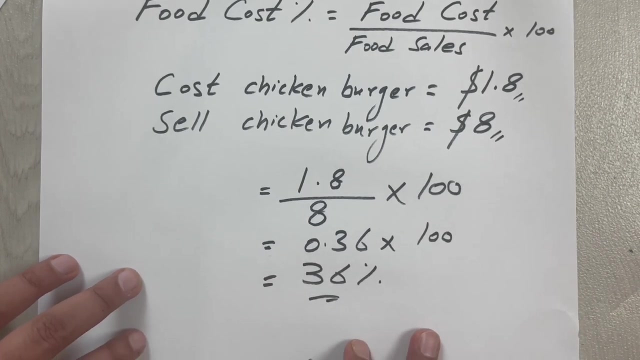 cost, then the food sale is 8, 1.8 divided with 8 multiplied with 100. so our answer is 0.36 when we divide this multiply with 100. so our answer is 36. so it means that 36 of the selling price.